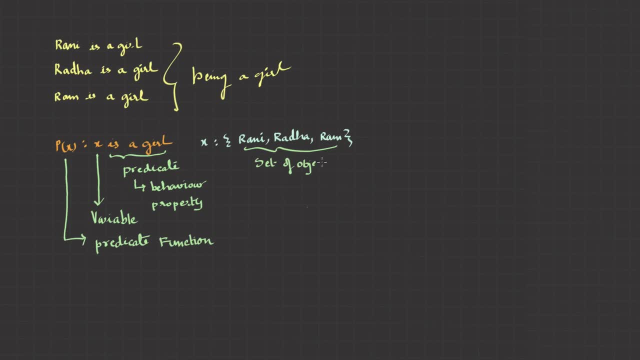 And this is a set of objects called the domain or universe of discourse. When we substitute the object in the predicate function, it becomes a predicate statement like this: These are instances or predicate statements which can be assigned with a truth value, But a predicate function is an open statement, so we cannot assign any truth value. 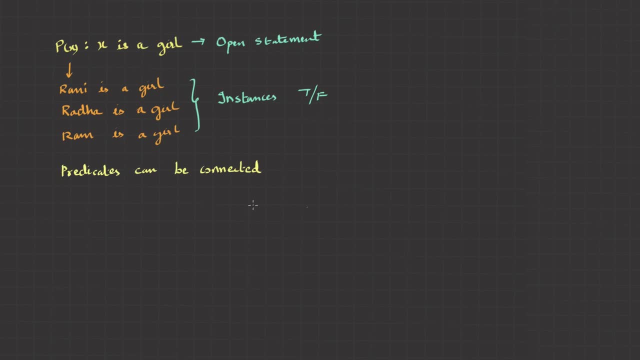 Similar to prepositions, even predicate statements can be connected with logical connectives like and or implication, etc. Here are a few examples. All these predicate statements follow the logical equivalence rules. Suppose I have a set x apples, oranges and mangoes And the predicate function is P- x is a fruit. 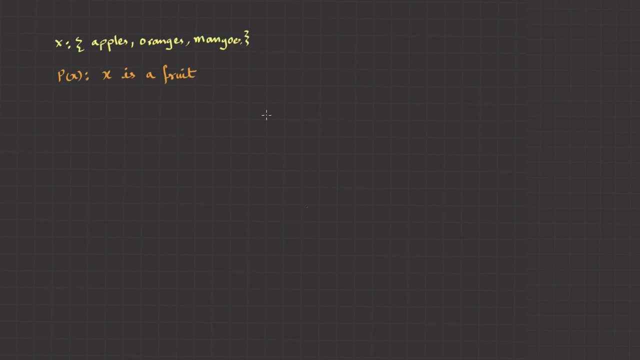 When we test this for every object, it always becomes true. Instead of writing each statement, I could write this as all are fruits. To denote this kind of statement, we shall use a special symbol For all. This is called a universal quantifier and we can read this as for all x, this becomes true. 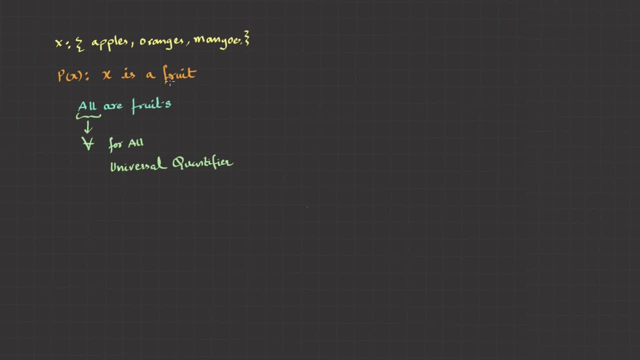 On similar lines for the set Y- apples, oranges, chocolate biscuit. I cannot claim that it's always true, but I can definitely say for some Y it is true, which I can write as some R fruits, This sum can be represented symbolically as this and read: as there exists some X which 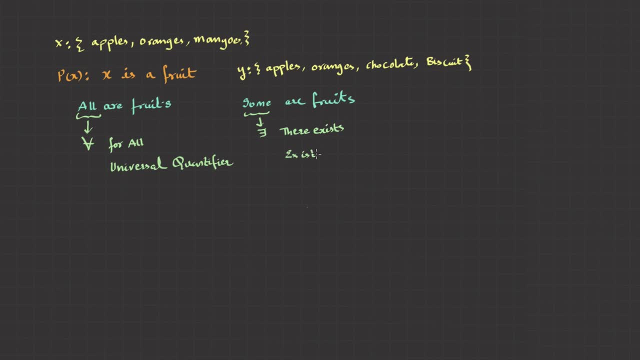 is true, This is called an existential quantifier. Now look at this. Every city in India is clean and the domain is city: Delhi, Hyderabad, Florida, Bay of Bengal. Now, if I want to put this in symbols, first I'll pick up the predicate functions C of X. X is a city in India. L of 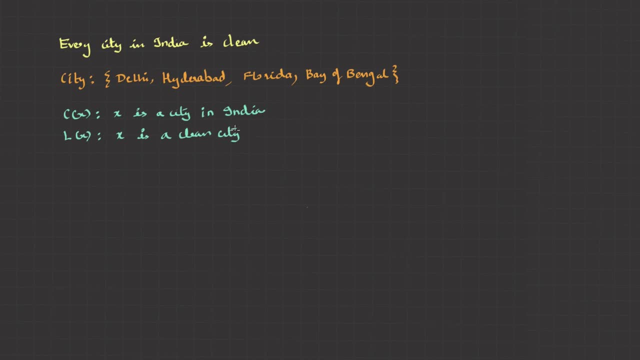 X. X is a clean city, then I can put it into symbols. as for all X, C implies L and it can be read. as for all X, if X is a city in India, then it is clean. now look at this: some days are holidays, days are Diwali. first Monday to my two, I can put it to predicate functions. 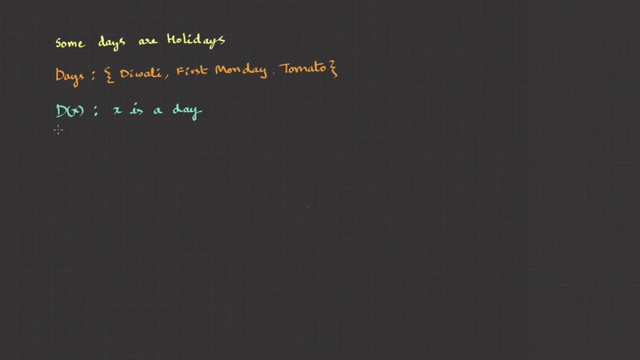 as D of X is X is a day, H of X is X is holiday, then I can put this into symbols as there exists X, D and H, and I can read it as there exists an X which is a day and it is a holiday. okay, so I can put it into symbols. as for all X, C implies L and it can be read as for all X. 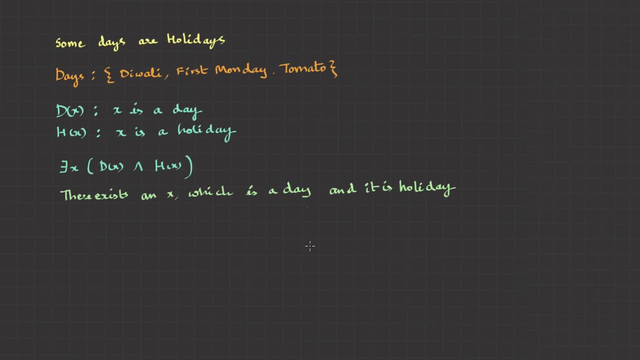 is a city in India. now you may have a doubt. why did we use implication in for all and conjunction in there exist? can't we use any other operator? the thing is, these are the only operators which satisfy in all conditions. let's introspect with the previous example. 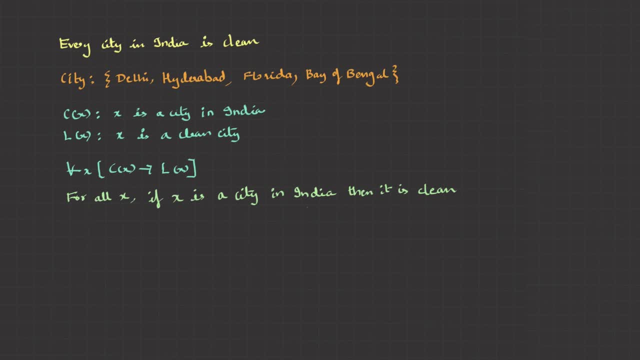 itself by swapping the connectives in for all. if I use and operator, it gives a meaning in there exists. if I use implication operator, it gives the meaning there exists an X. if X is a day, then X is holiday. thus fails for tomato, as tomato is not a day and it is not. 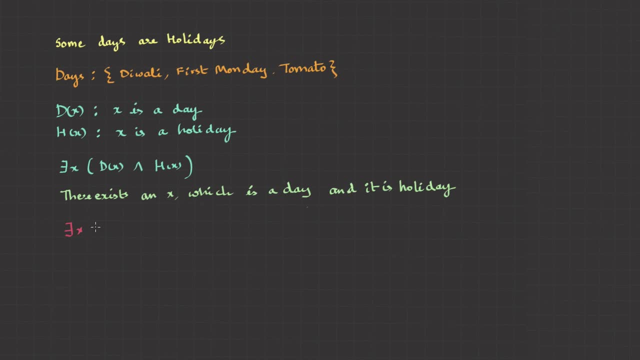 a holiday. false implies false is true if you use implication operator it way to get a point. two, as for all X, for all X, D and X is clean. for all X. they are the other operation that agree on skin is become ugly. or that says don't care about system cause you cannot useül. 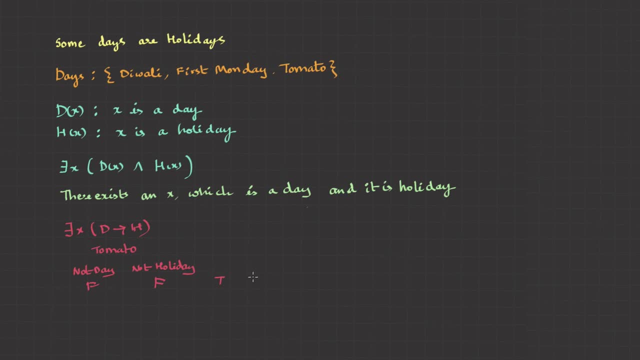 So if you run this in a machine with implication operator, then machine says tomato is accepted for holiday because it's becoming true, which is actually wrong. So for all is always associated with implication and there exist is always associated with conjunction. Blindly remember this. it's very, very important.